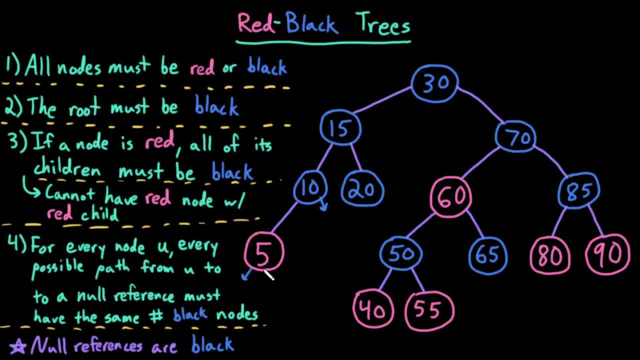 To the right. 5 has two null references, left and right. 20 has two null references, So I'll just go ahead and fill these all out. So all of my leaves have two null references, a left and a right. It's something that could have been a child but is currently null. 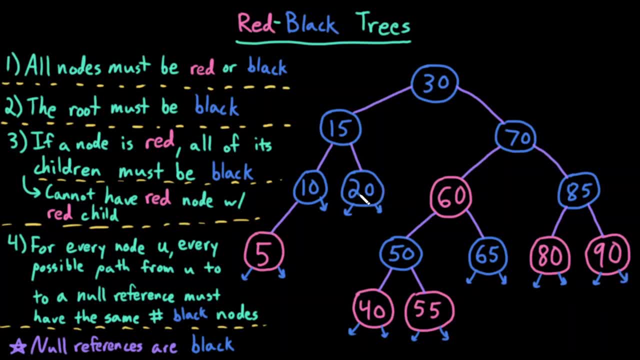 And then elsewhere in the tree it's something that could have been a child but is currently null. So 20 was also a leaf, 10 had a null right child And it looks like nothing else in the tree has any null children that I haven't already marked. So, other than leaves, the only one that had, 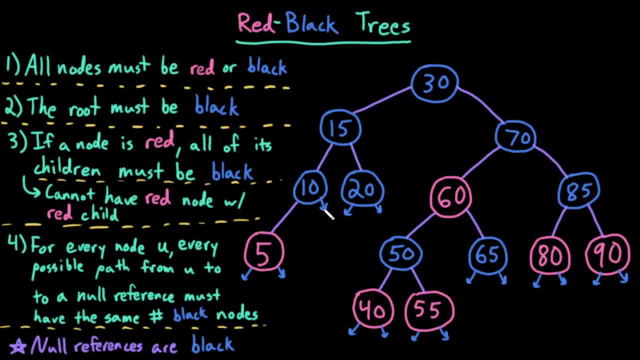 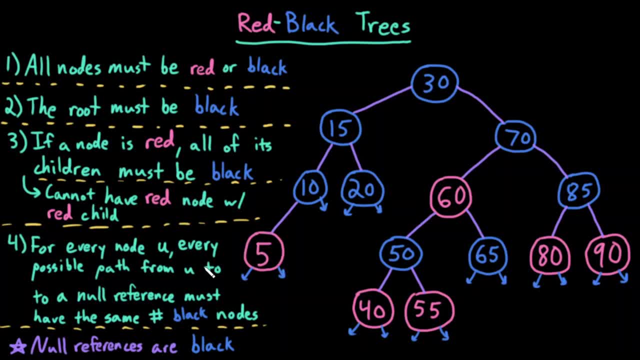 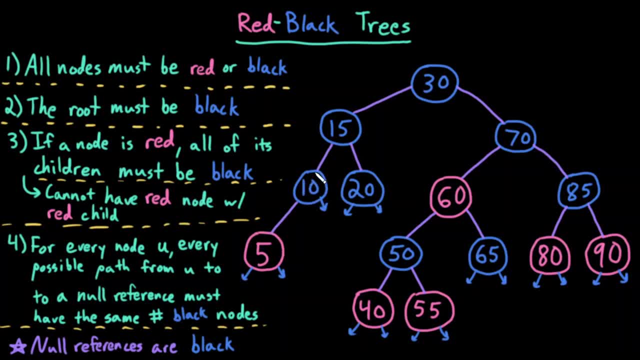 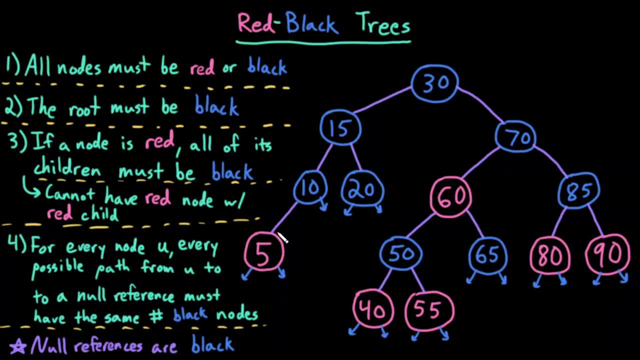 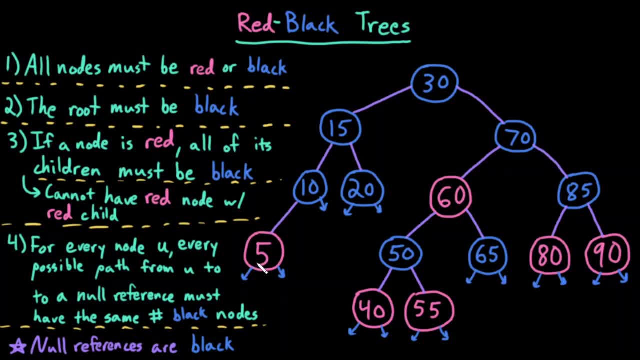 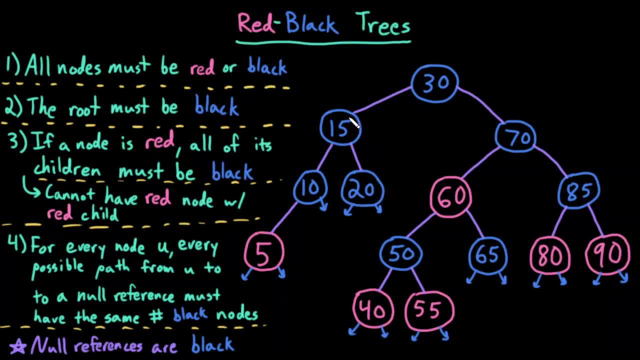 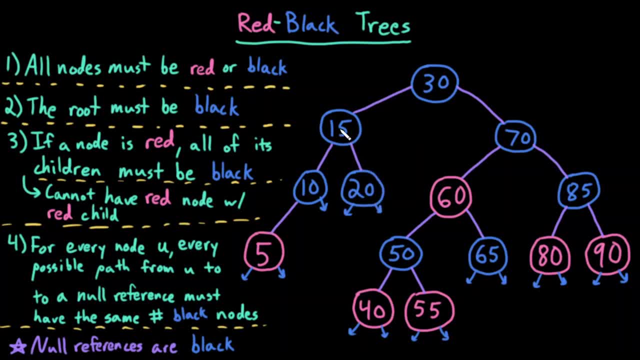 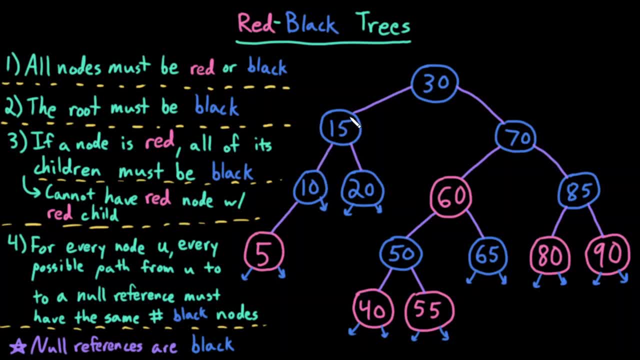 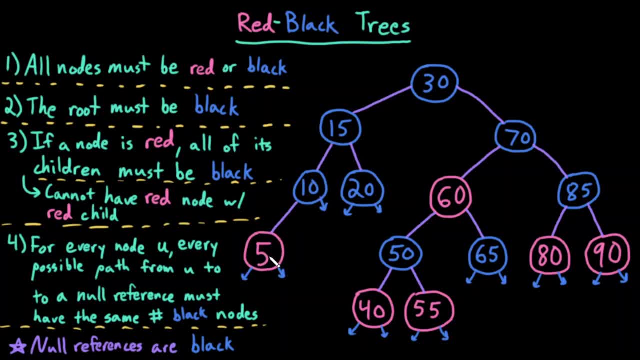 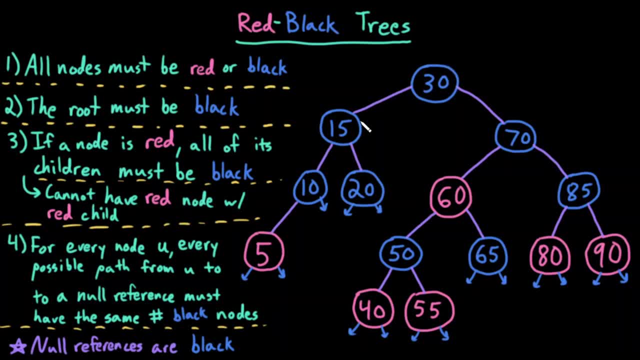 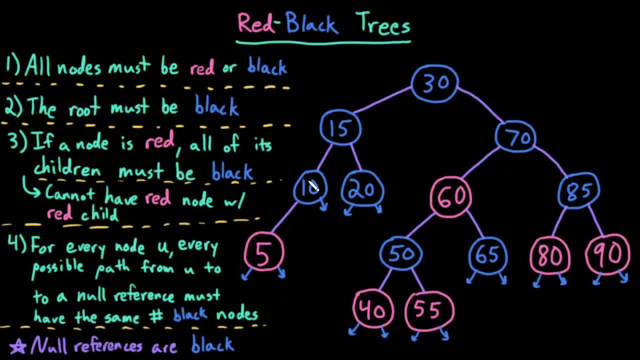 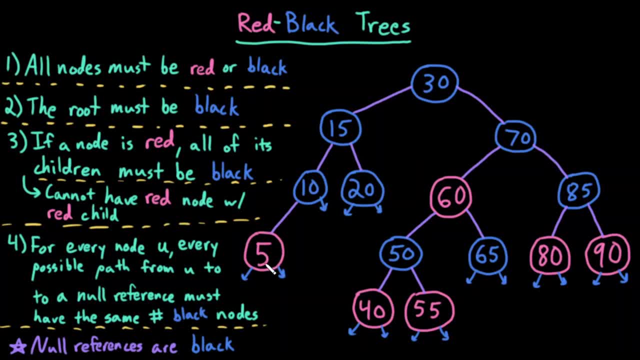 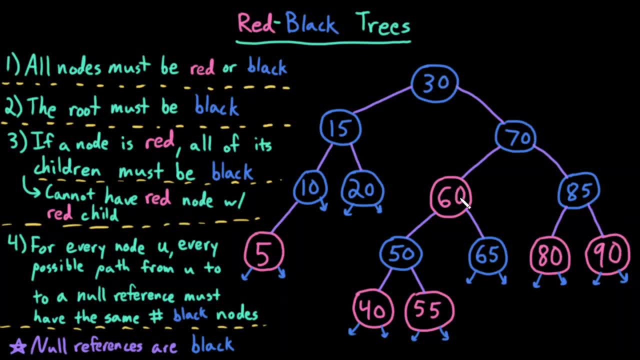 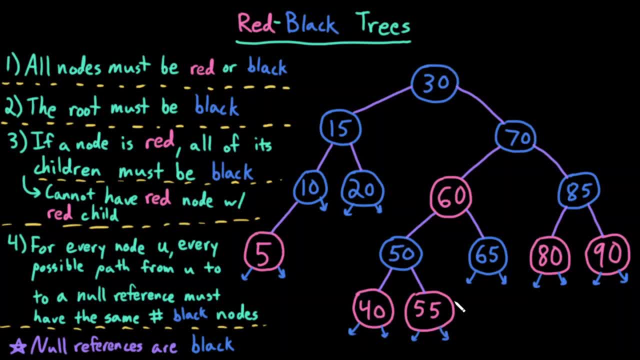 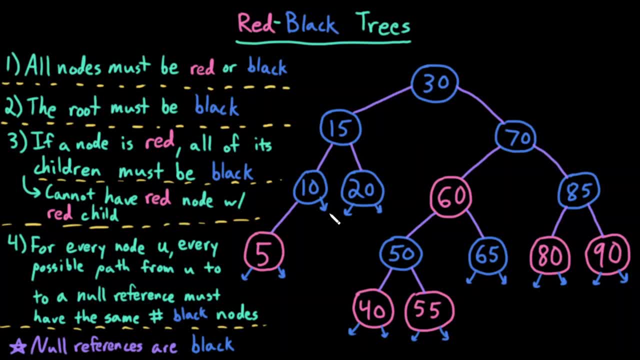 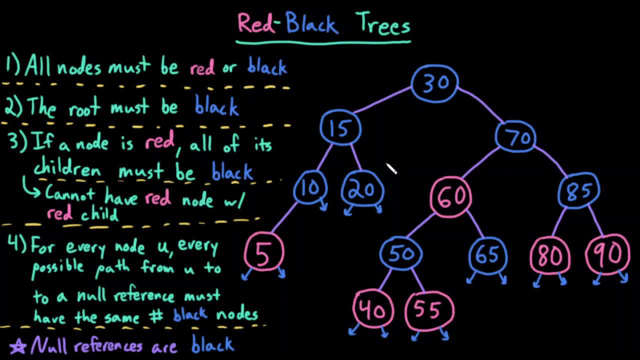 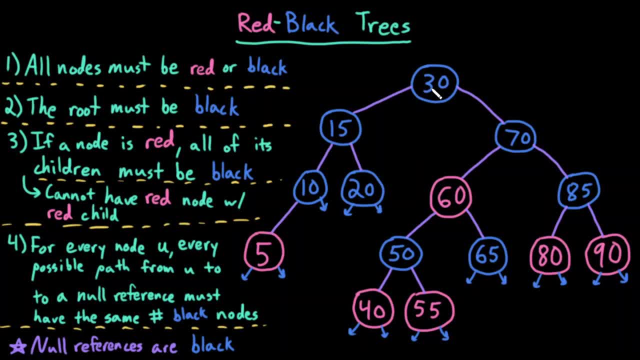 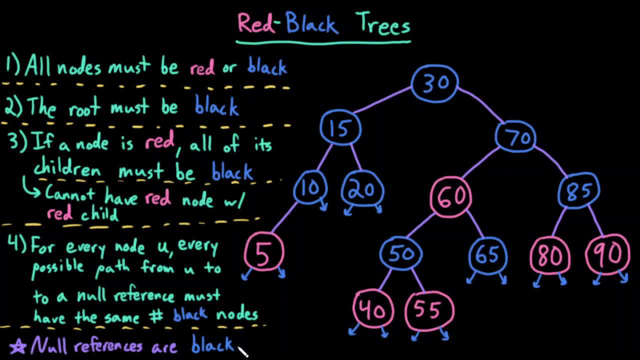 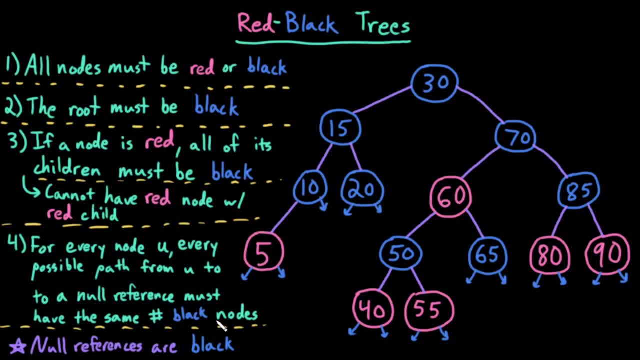 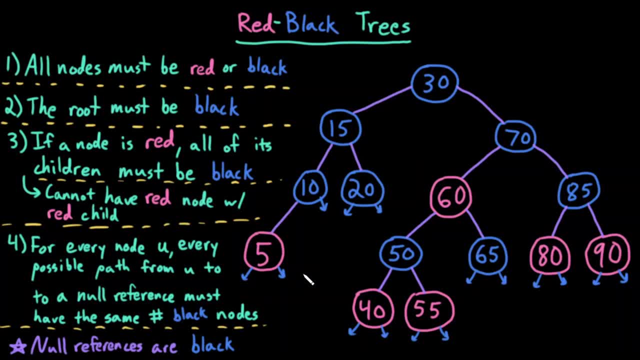 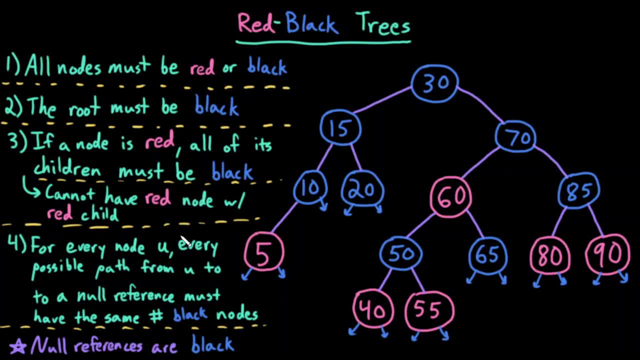 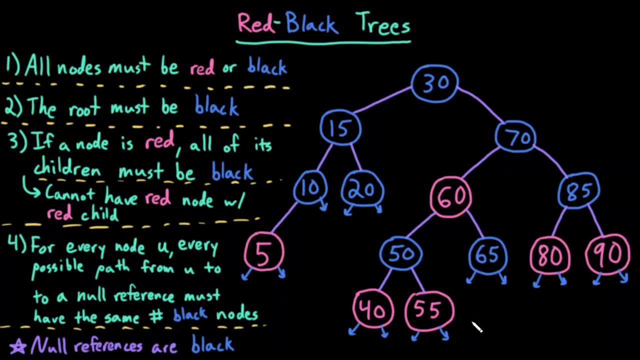